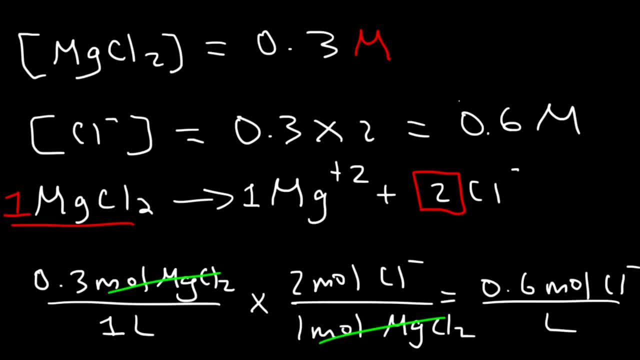 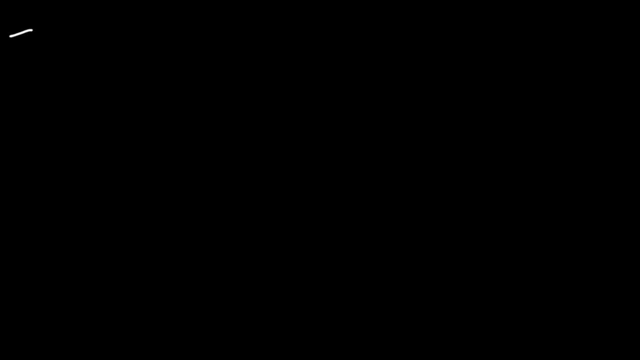 moles of chloride per liter of solution, which equals the concentration of MgCl2.. correlates to a concentration of 0.6m. Now let's try some more examples. So let's say that the concentration of aluminum chloride is 0.20.. So, given this information, what is? 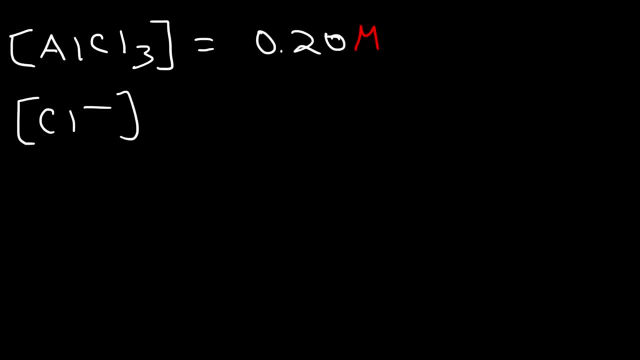 the concentration of the chloride ion in the solution. Feel free to pause the video and try this problem. The quick and simple answer: it's going to be 0.20 times the subscript 3.. So it's going to be 0.60.. Now here's another one. Let's say, if we have the concentration, 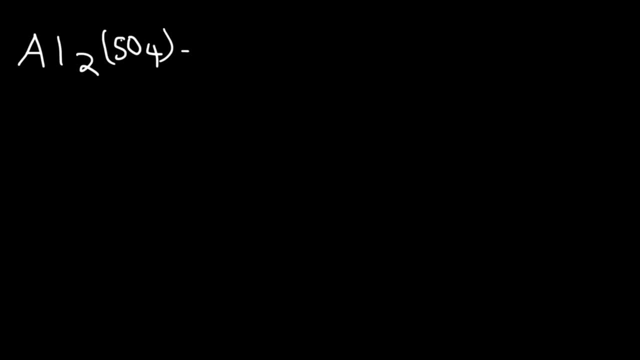 of aluminum sulfate, Let's say it's 0.15 moles per liter. So with this information find the concentration of the aluminum 3 plus cation and of the sulfate anion. So for the aluminum cation it's going. 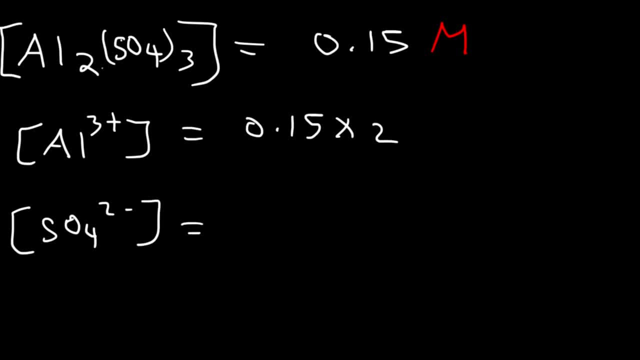 to be 0.15 times 2, because we have a subscript of 2.. So that's going to be about 0.30m, And for sulfate we have a subscript of 3.. So it's going to be 0.15 times 3, which is 0.45m. 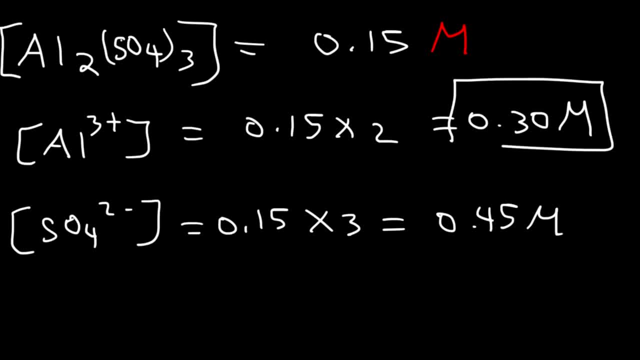 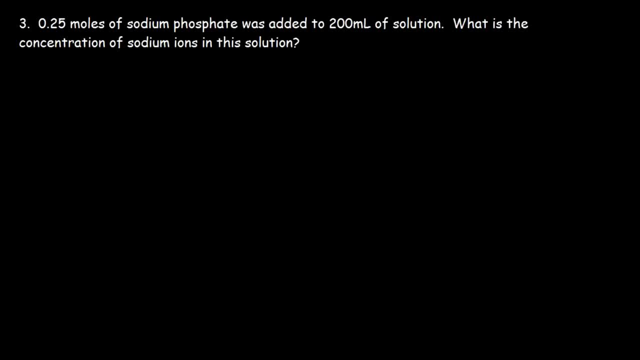 So that's going to be 0.45m, And so that's a quick and simple way of how to calculate ion concentration from molarity. Now let's work on some more problems. 0.25 moles of sodium phosphate was added to 200. 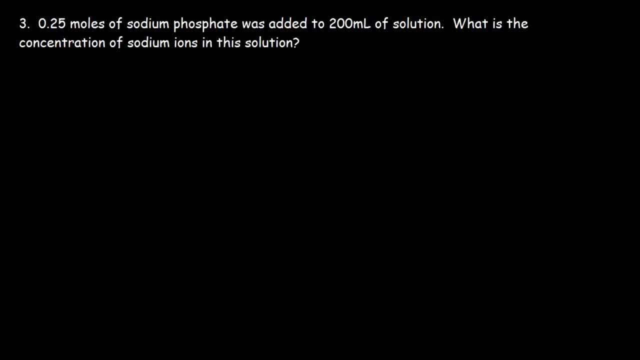 ml of solution. What is the concentration of sodium ions in the solution? So first we need to calculate the concentration of sodium phosphate. To find the molar concentration, or the molarity, we're going to need a molecule called pt2.. In this molecule we're going 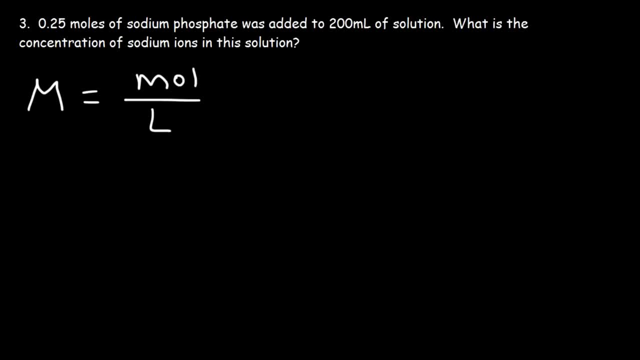 to need a molecule that is 2 mol of sodium, So we're going to use one molecule of sodium. One molecule is a concentration of sodium, So we're going to use one molecule of sodium. we need to take the moles and divide it by the number of liters, so we have 0.25 moles of sodium. 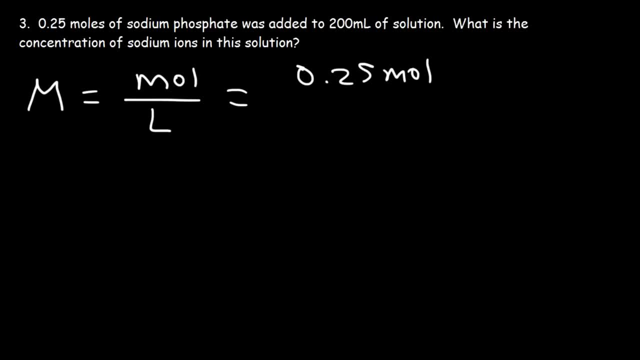 phosphate. now, what is the formula of sodium phosphate, because that's important. sodium has a positive one charge. it's an alkali metal in group one. phosphate is po4, three minus. so, using this crisscross method, it's going to be na3 po4. now, having the one there is, there's. 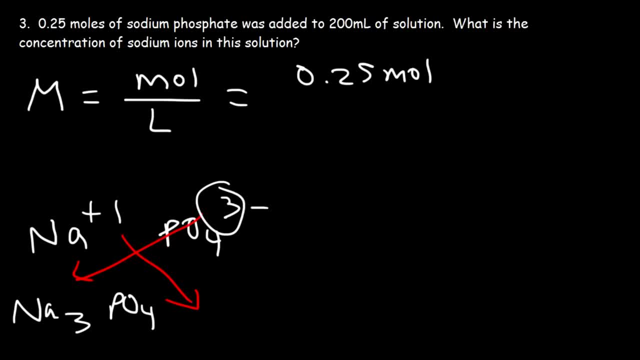 no point. so you don't need to write the one, but the three. it's important. you need to put in front of na. so we have na3 po4. that's the formula for certain phosphate. now the next thing we need to do is convert milliliters into liters. now recall that one liter is equal to a thousand milliliters. 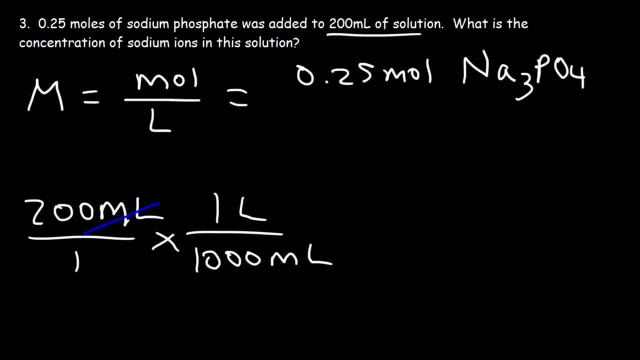 so you got to divide by a thousand when you convert. you want to convert in such a way that the unit cancels. 200 divided by a thousand is 0.2. so we're going to take 0.25 moles and divide it by 0.25 liters. 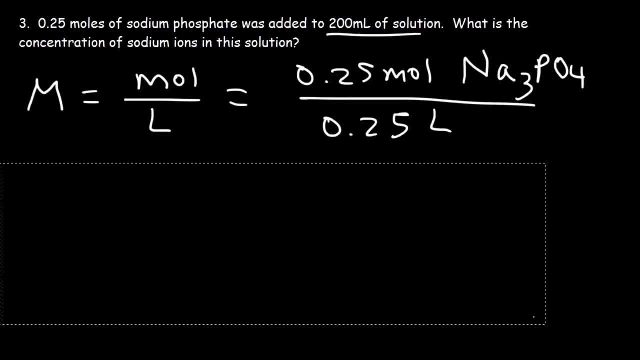 so let's use the calculator to do that. and that's not supposed to be 0.25, that's supposed to be 0.2 liters. 0.25 divided by 0.2 is 1.25. so this is the concentration of sodium phosphate. 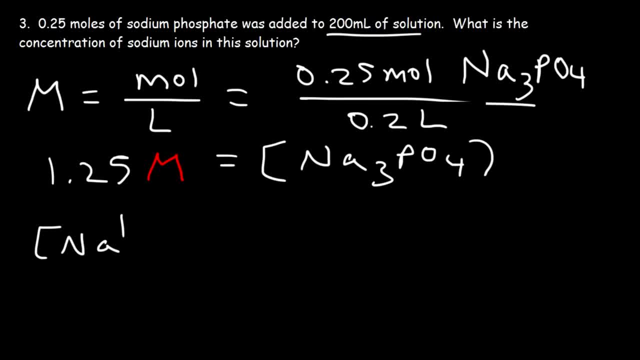 so now that we have that, we could find the concentration of the sodium plus cation. it's simply going to be 1.25 times 3 based on this number, so that's about three times three, so that's about 3.75. so here's a new problem that we could try: 600 milliliters of water. 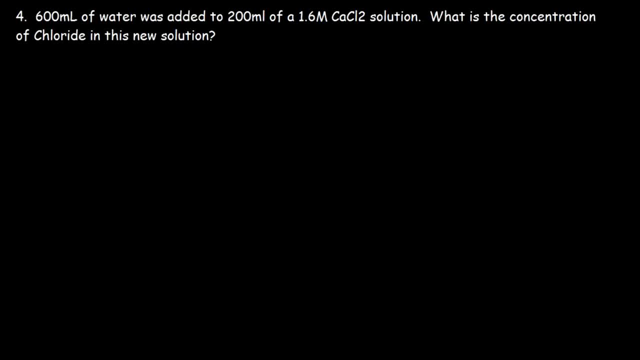 was added to 200 milliliters of a 1.6 molar calcium chloride solution. what is the concentration of chloride in this new solution? so what we have here is a dilution problem. whenever you add water to a solution, the volume increases and the concentration decreases. 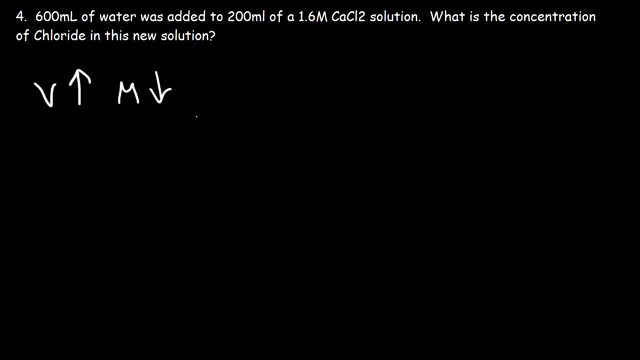 or we could say the molarity decreases, and for this type of situation you could find a new concentration using this formula: m1 v1 is equal to m2 v2, so the original concentration of calcium chloride was 1.6 m and the original volume was 200 milliliters. 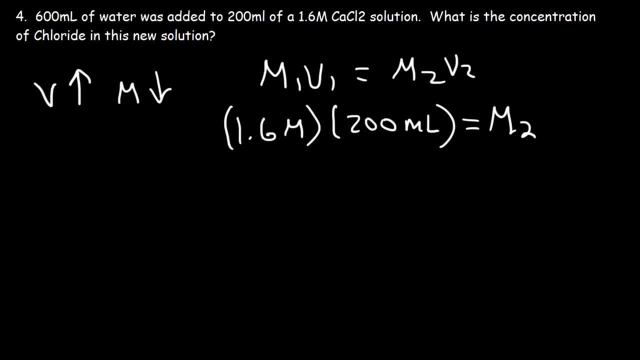 now our goal is to find a new concentration. if we could find the new concentration of calcium chloride, then we could find the concentration of the chloride ions in a new solution. now, what is v2? what is the volume of the new solution? we started with 200 milliliters of calcium chloride solution. then we've added 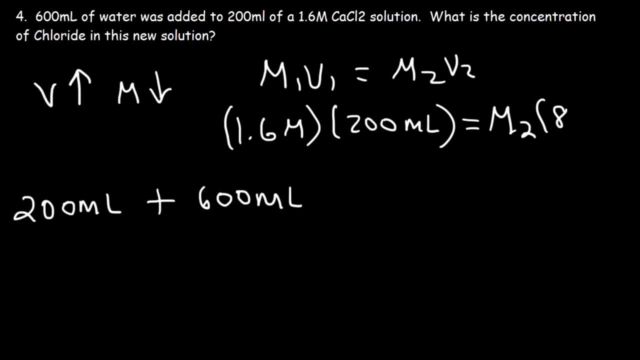 600 milliliters of water, so now the total volume is 800 milliliters. now let's go ahead and calculate the new concentration. so it's 1.6 times 200, which is 320, and then take that divided by 800, so the new concentration is 0.4, that's m2. so the concentration of calcium chloride 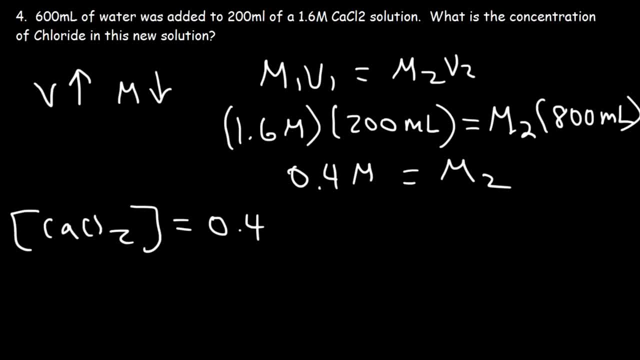 in the new solution is 0.4 m. now we can use that to find the concentration of the chloride ions. it's going to be 0.4 times 2, based on this subscript. 0.4 times 2 is 0.8 and so that's the. 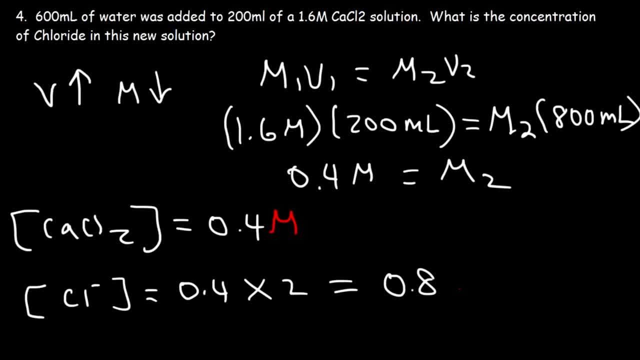 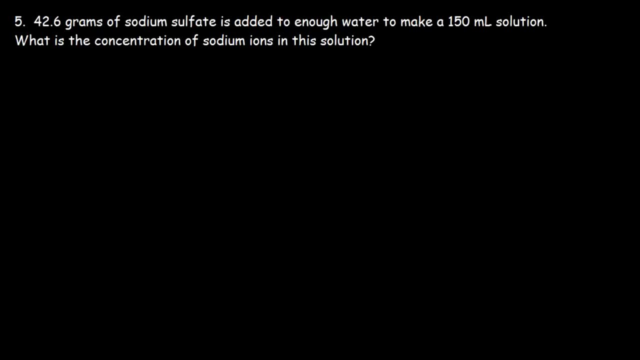 answer for this problem: for every liter of solution there's 0.8 moles of chloride. try this problem. feel free to pause the video as you work on it. 42.6 grams of sodium sulfate is added to enough water to make a solution that is 0.8 moles of chloride. 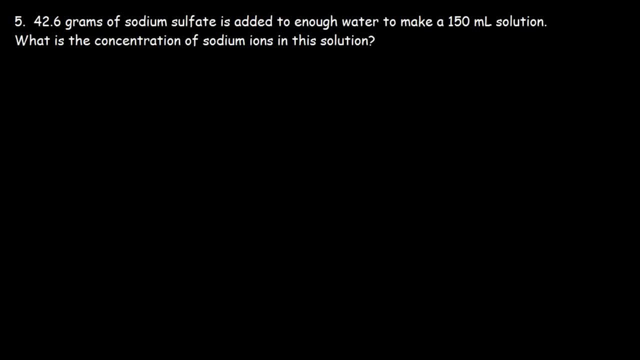 so that's the answer for this problem. to make a 150 milliliter solution, what is the concentration of sodium ions in this solution? now, the first, most important thing that we need to do is write the correct formula of sodium sulfate, because if we mess up in this step, the entire problem is gone. we're not going to get it right. 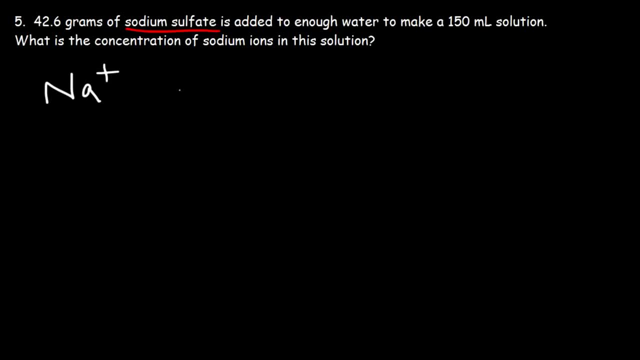 sodium has a plus 1 charge. sulfate is a polyatomic iron, that's so4 2-. so make sure you know you're adding sodium. sulfate to your solution is 0.1, much less than same amount of sodium. that's why so42- so make sure you know you're adding sodium. 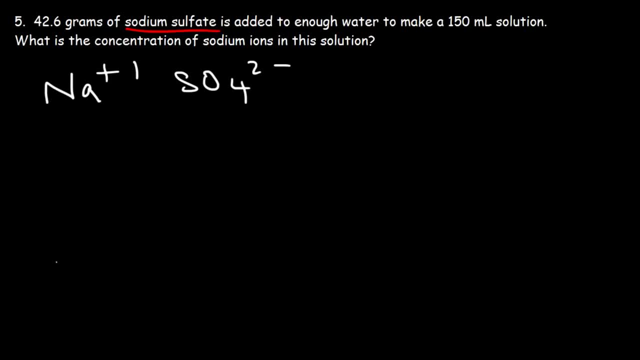 your polyatomic ions. Now to write the correct formula, we're going to turn the plus one charge into a subscript and the minus two charge into a subscript, So it's going to be Na2SO4 times one. If it's a one, you don't need the parentheses. If it's two or more, you do need it. 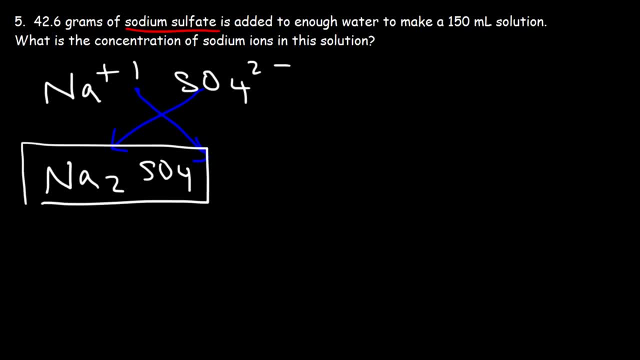 So this is the formula of sodium sulfate. Now that we have that, let's find the molar mass. That's the next thing that we need. So we have two sodium atoms, one sulfur atom and four oxygen atoms. The atomic mass of sodium is 23,, sulfur is about 32, and oxygen is 16.. So we have 46 plus 32. 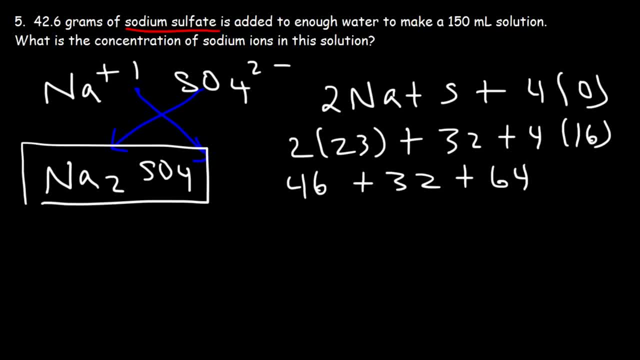 plus 64.. 32 plus 64 is 96.. 96 plus 46 is 142.. So the molar mass is 142 grams per mole. Now let's start with 42.6 grams of Na2SO4.. Let's convert it to moles. So one mole of sodium sulfate has a mass of 42. point, or rather 142. 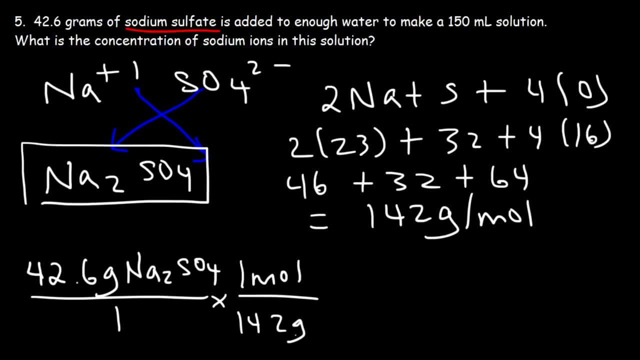 grams. That's the molar mass And I'm going to write the substance. I already have: Na2SO4.. SO 4 is equal to NOTYOUNABLE, So notice that the unit grams cancel. So now we have moles of sodium sulfate. Now I'm gonna convert it to moles of sodium ions. 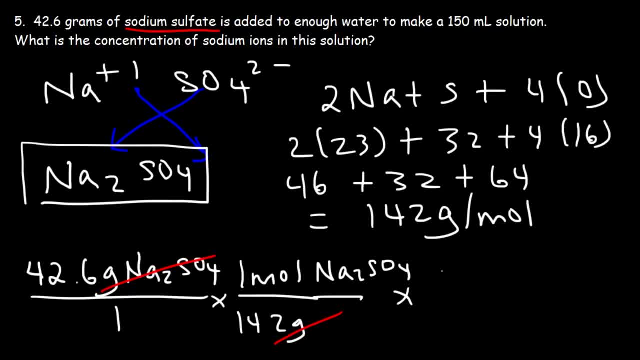 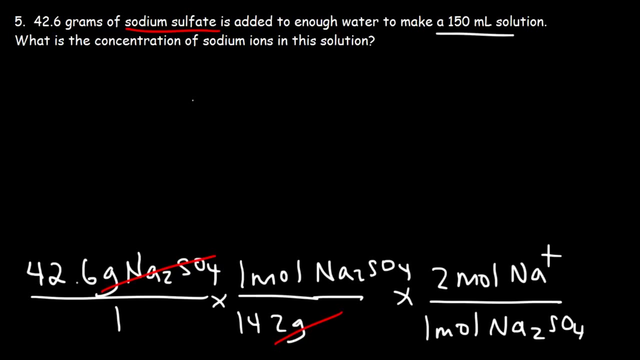 Notice that there's two sodium ions per formula unit, so there's two moles of Na plus for every one mole of Na2SO4.. now we know how to convert 150 milliliters into liters. as we've done before, we divided it by a thousand, so 150 milliliters multiplied by 1 liter. 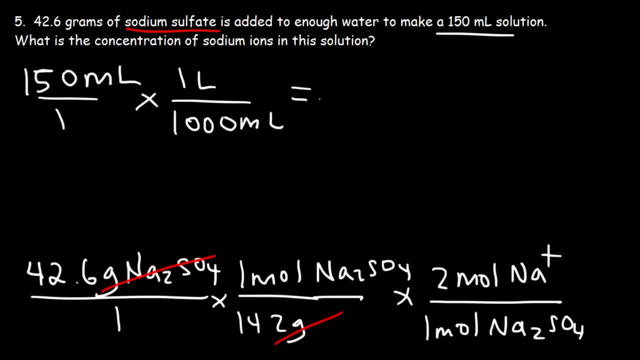 per thousand milliliters. this is equal to 0.15 liters. these units cancel. so to get molarity we reduce it, divide by .15 liters, so moles of sodium sulfate cancelled. so now we have moles of Na plus ions over liters, and that will give.